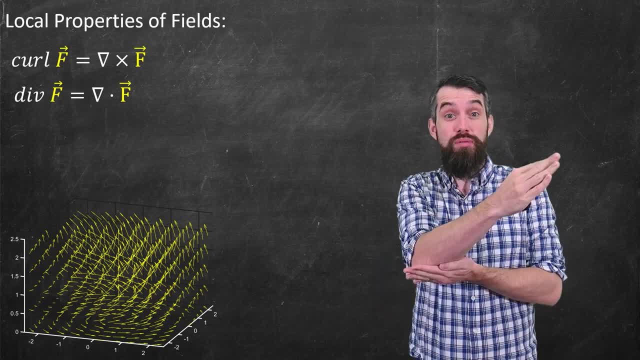 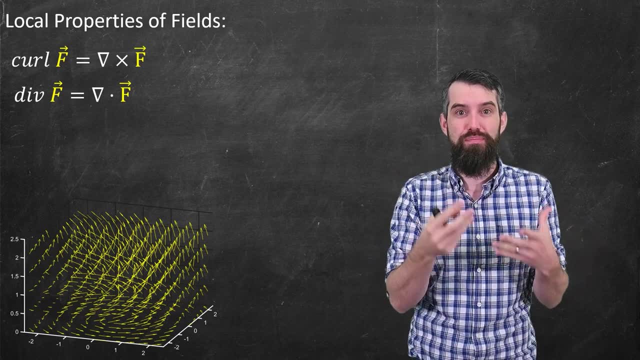 Curl gave the tendency for the field to sort of spin around some particular axis and the divergence gave the tendency of the field to be separated away from some point in a nearby region of that point. Both of these are local properties. We can contrast that with some. 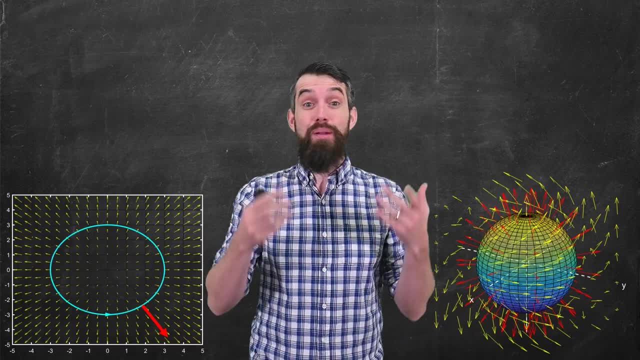 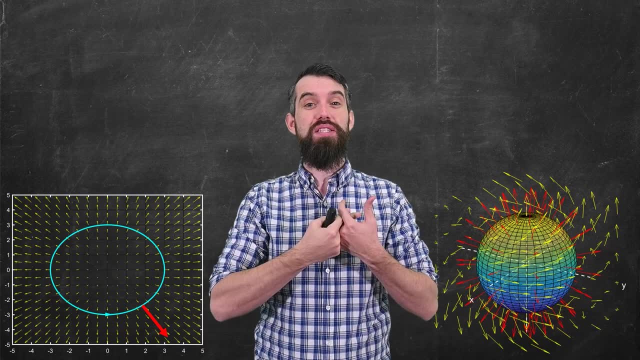 global properties that we've seen in vector calculus, For example. I'm going to put up a two-dimensional and three-dimensional pictures of the same story. In the two-dimensional case, I'm trying to figure out the flux across a particular curve, the tendency for the field to leave the 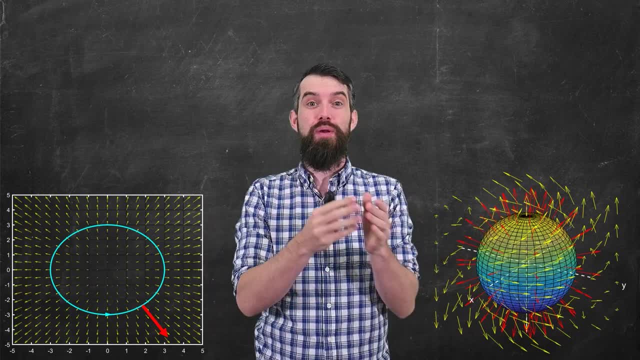 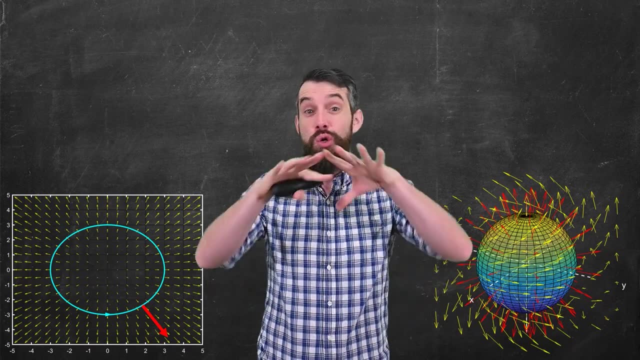 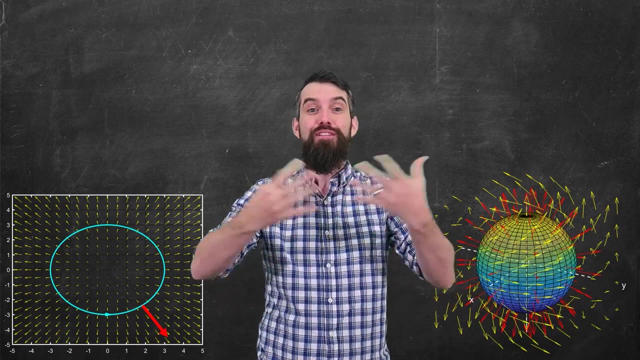 curve, In other words, the tendency for the field to be aligned with the normal vector to the curve. The same story is true in three dimensions. If I have a closed surface and I have normal vectors leaving from that surface, the question is, to what degree is the yellow vector field f leaving or 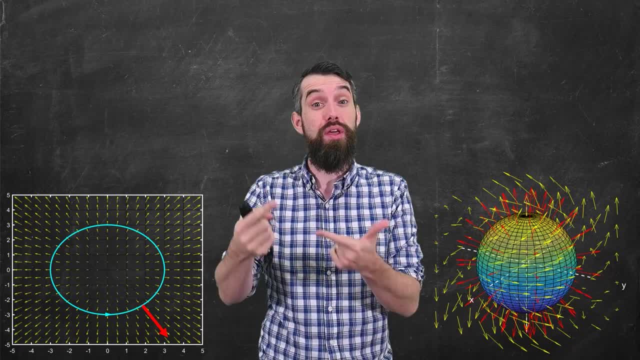 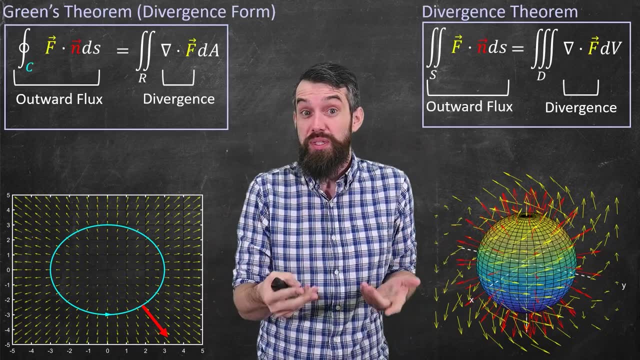 spreading out across that surface, in other words, aligned with the normal vectors. These are global properties. they're about entire curves or they're about entire surfaces. And then the two theorems we saw about outward flux was Green's theorem in its divergence. 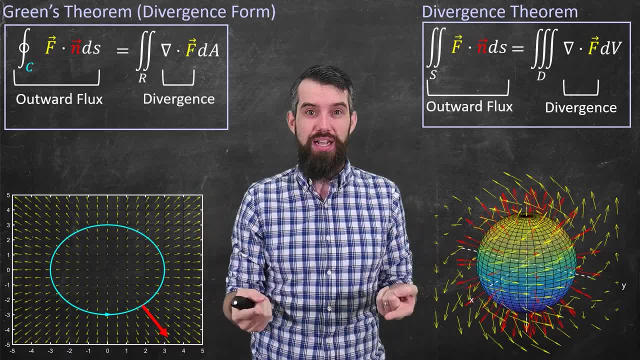 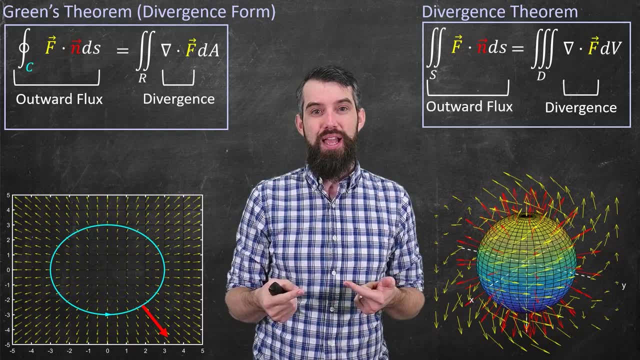 form and the divergence theorem. Both of these computed the outward flux. In Green's theorem it's the outward flux across a curve and in divergence theorem it's the outward flux across a surface. And then what's core about these is that this property around the boundary, what I'm going. 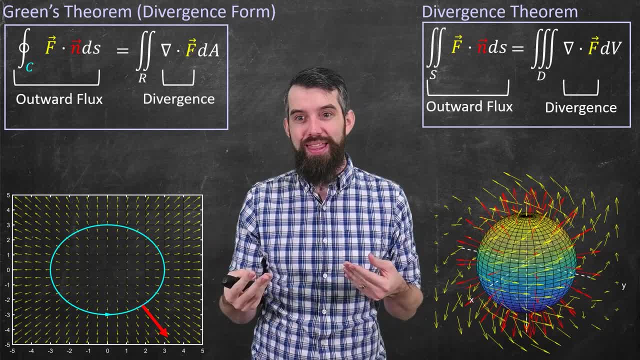 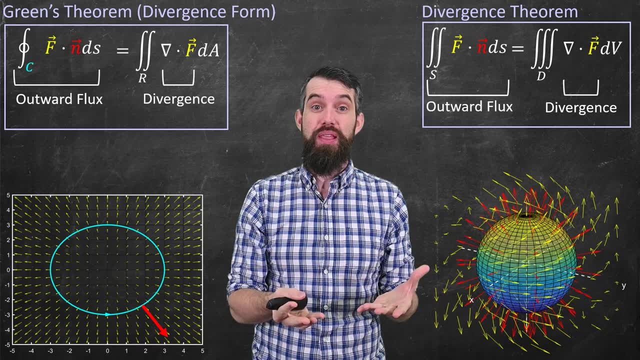 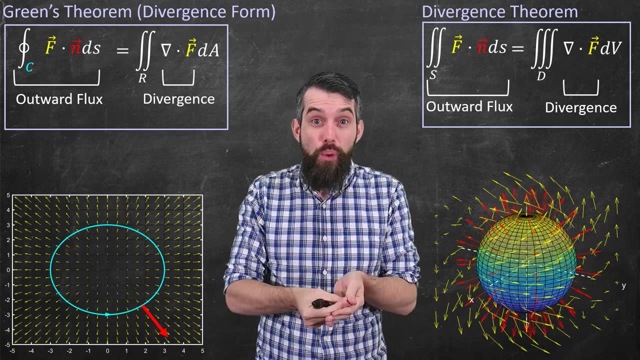 to call a global property could be equated with adding up or integrating a local property of the divergence throughout the entire region. So in the case of Green's theorem, the region is some area and if you add up all those local properties, the divergence at every point inside of the domain, you get the global property. 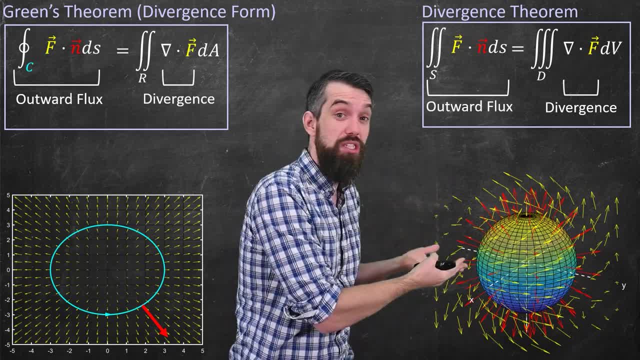 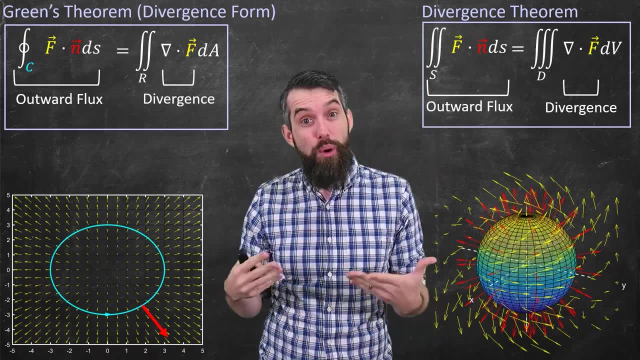 of the outward flux across the boundary. Similar for the divergence theorem. your closed surface now encloses a volume and if you add up that local property of the divergence at every point in the volume, it's going to add up to the global property. 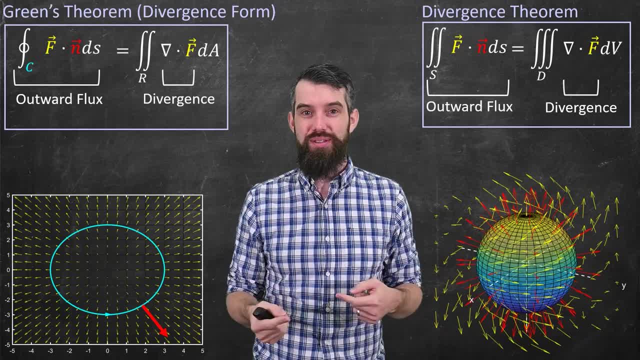 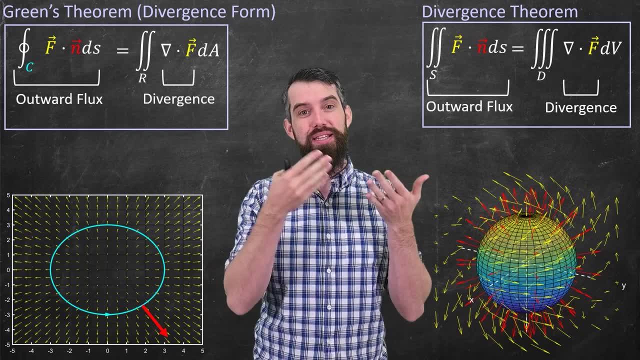 of the outward flux across the boundary of that region. So the key takeaway here is that this accumulation on a boundary could be expressed as adding up a local property, in this case the divergence. So the divergence of F was one of our so-called differential operators on F. 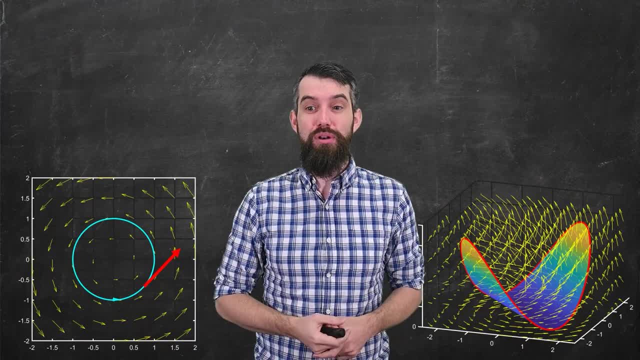 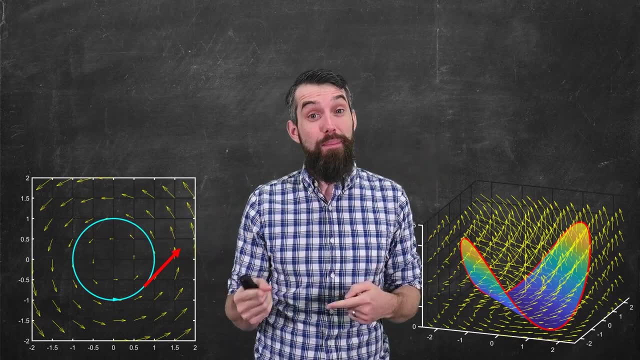 But we had a different one, which was given by the curl. We have a similar story there, So we have a two-dimensional case and a three-dimensional case. In the case of the curve, we're now trying to measure the circulation, which is the tendency. 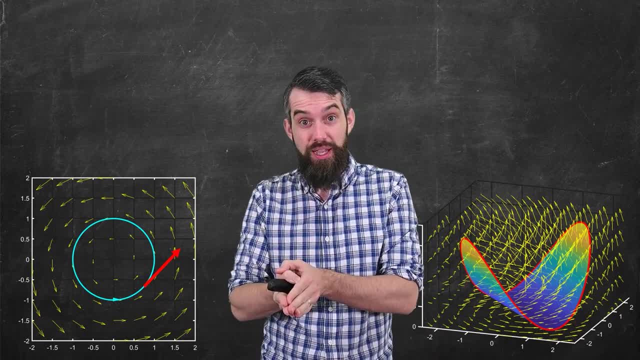 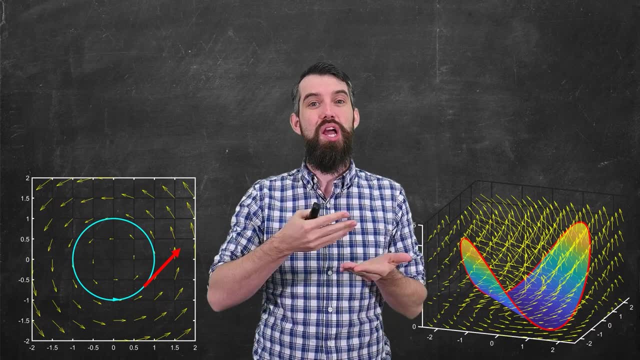 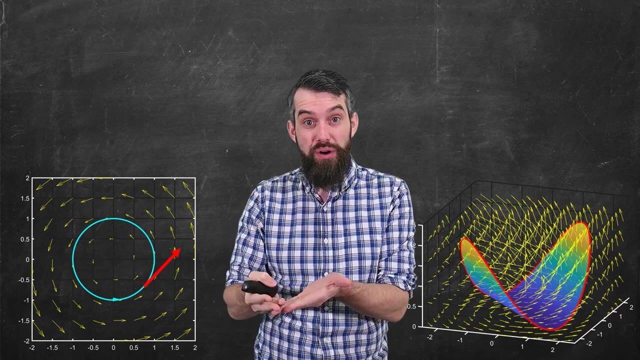 for the vector field to be aligned with the tangent vectors And similarly, if we go to the three-dimensional situation, you could have a surface that has a boundary curve and we're asking: what is the tendency for the vector field to be aligned with the tangent vectors to that boundary curve? 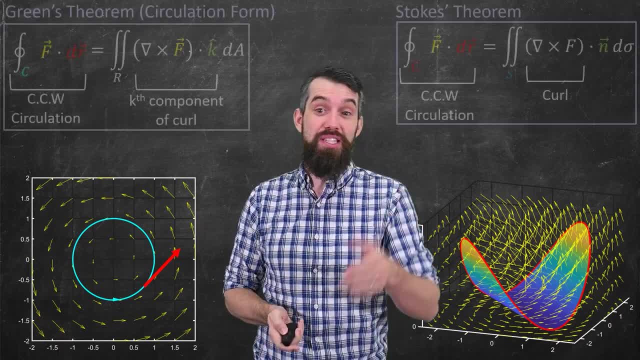 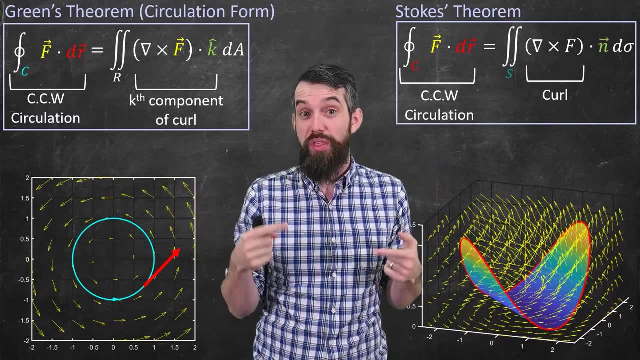 And, just as with the Green's theorem and the divergence theorem, we have a similar relationship with the other three-dimensional case: The other half of Green's theorem, called its circulation form, and Stokes' theorem, And they're both talking about the counterclockwise circulation, either just around the curve. 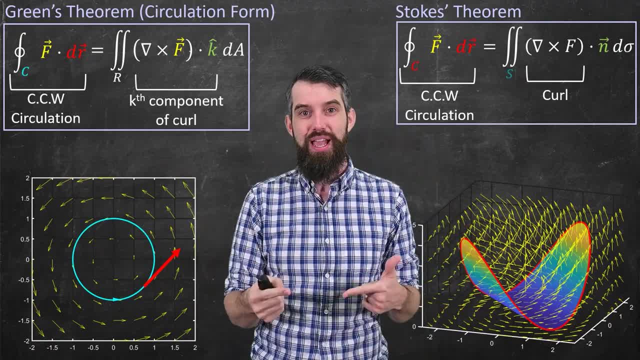 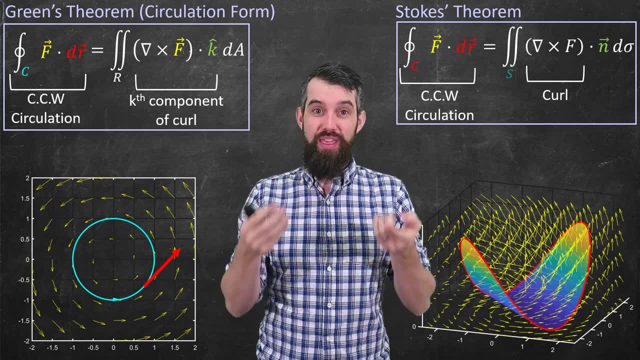 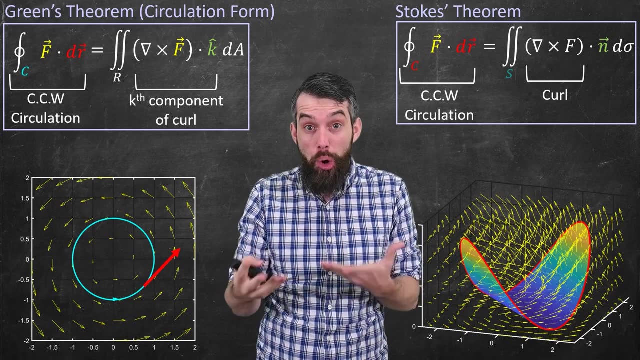 in two dimensions or around the boundary curve of your surface. And really what they say is again, this property around the boundary can be written as adding up the local property of the curl or K-th component of curl, for just in two dimensions, But either way, adding up this local property over the entire domain. So in the case of Green's theorem we have a three-dimensional case And again this property around the boundary can be written as adding up the local property of the curl or K-th component of curl, for just in two dimensions. So a three-dimensional case can be written as adding up the local property of this visualization. And the five-dimensional case is made up of this degree. so in total, within the plane form that we look at, that's justточно as that example starts to occur. So let's look at the same principle again that we just say: lets us stop playing with K-th. and add up the grade documentation for this final equation, We see again that if we want to get rid of this perimeter, we have to add aib, which is a positive preference, and the negative preference is give it anti-directional value. 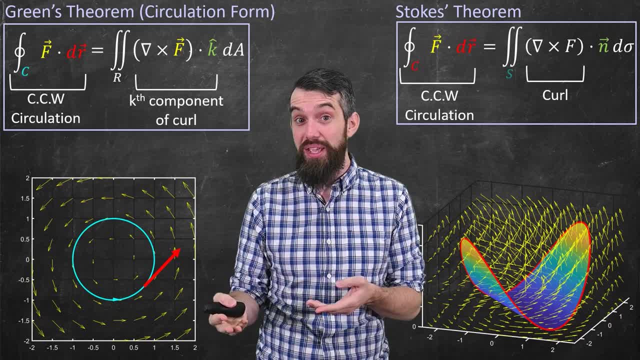 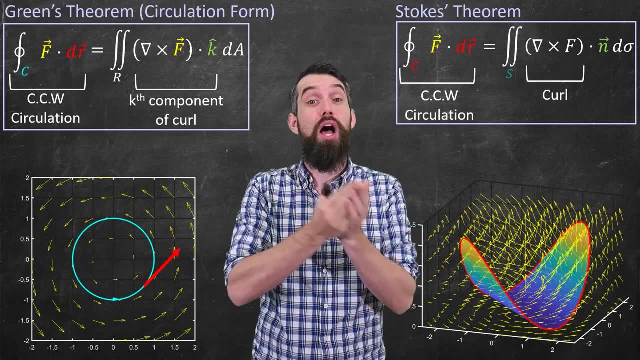 upon its conservation And ultimately we're wrong, We're not going to get a range of dimension over these three dimensions. So then we'll have this line and we can't face it at all. Here to all, this found simple and only the first machine which has an enterprise of its own, a fixed cell which 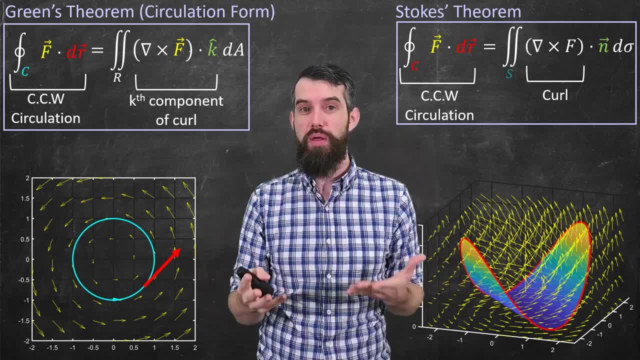 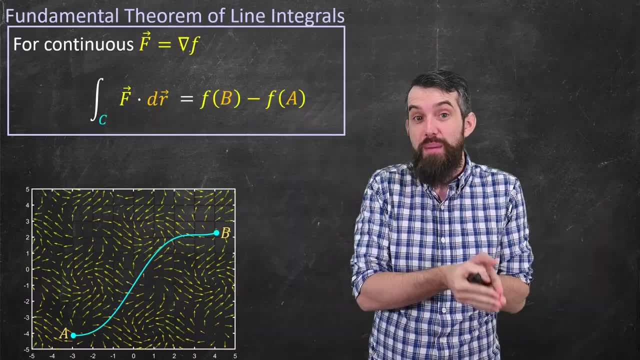 over the entire domain gives us this property along the boundary. Okay, so let's see how far this pattern goes back, because we actually saw a little earlier in the course something called the fundamental theorem of line intervals. This was a measure of the flow along a curve. 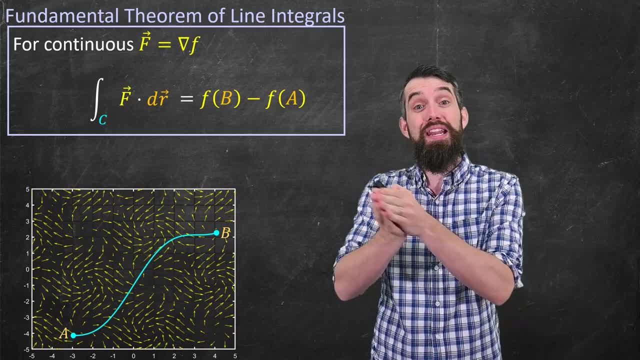 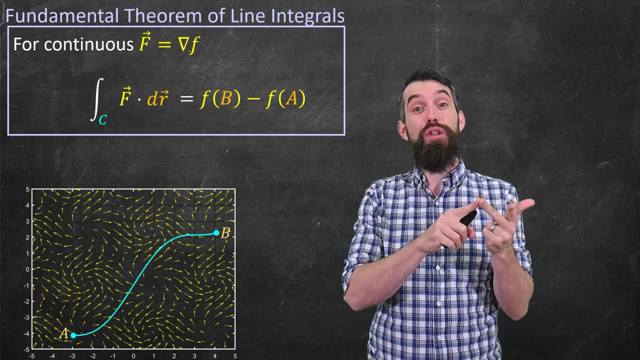 but it was specifically for when you had a vector field that could be written as the gradient of f. We've had the divergence of a field, we've had the curl of a field and now we have this third thing, when a field is written as the gradient. 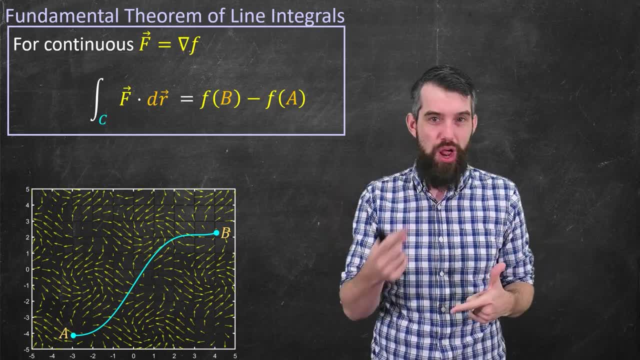 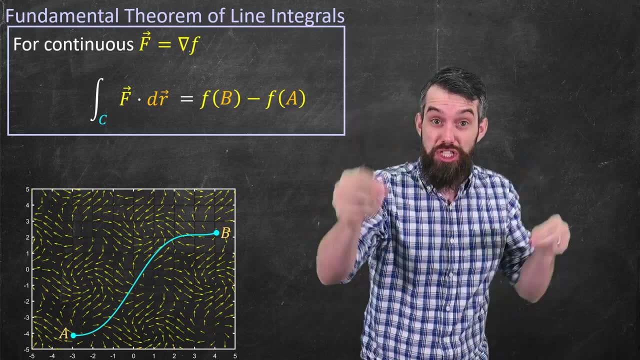 of a scalar potential function. It's sort of a different type of differential operator, a differential operator on the scalar potential function now. Now, the boundary of a curve that has n points is just well, just the two points, those two n points. 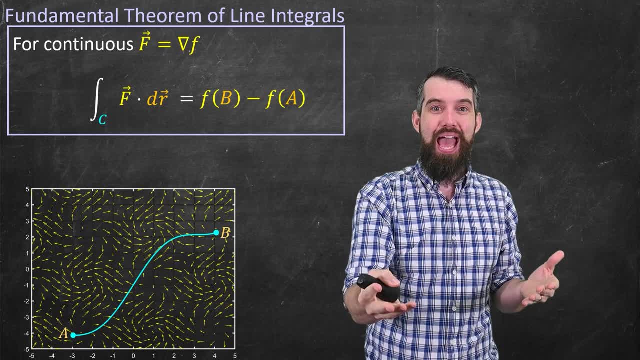 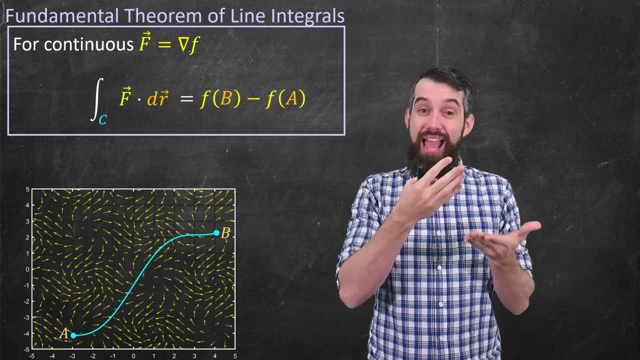 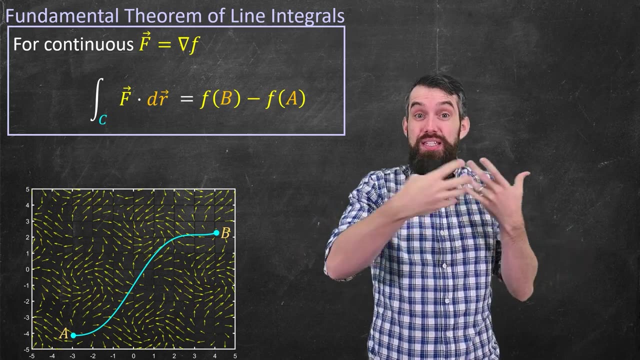 The boundary is a little bit simpler And yet once again we have a similar kind of local to global transition When you integrate a differential operator. so in this case we're integrating the gradient of f and we integrate that over the entire region. 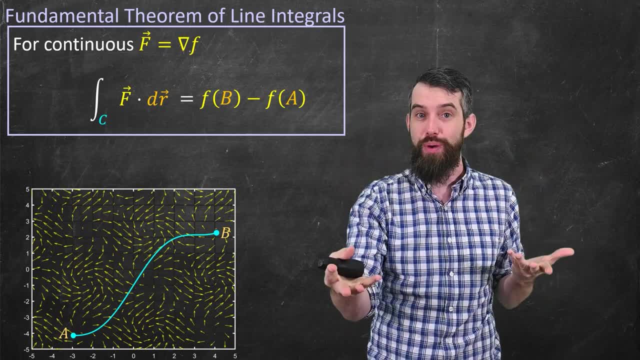 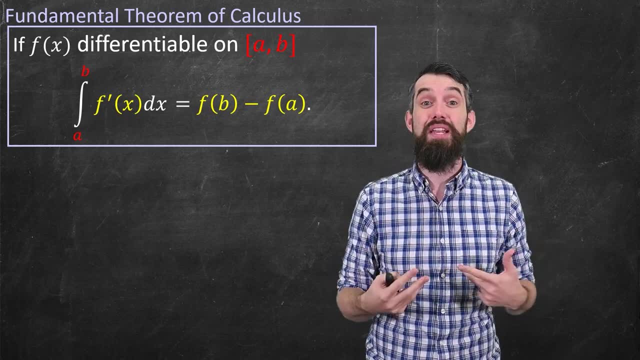 you just get some result on the boundary, in this case the two n points, f of b minus f of a, And this could be pulled back even further to the fundamental theorem of calculus 2, which said that you have a differentiable function. 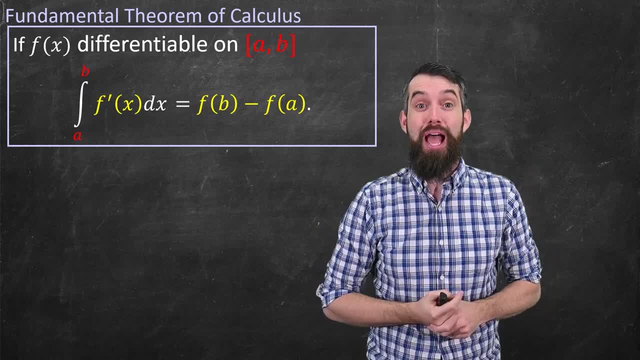 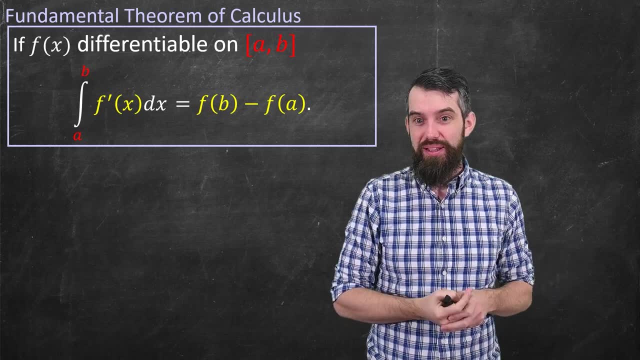 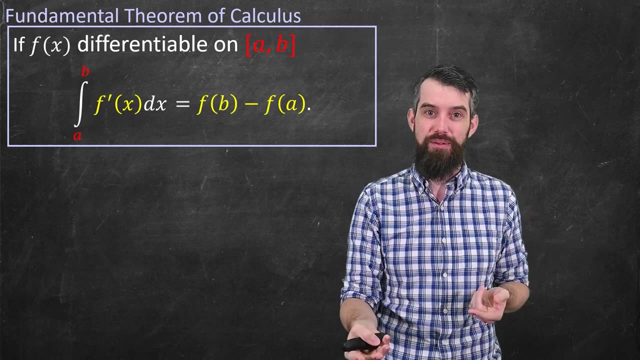 when you integrate the derivative. The derivative is perhaps the simplest of these so-called differential operators, something that acts on a function by taking some type of derivative. Then the integral of this derivative is just some information about the boundary points, only: f of b minus f of a. 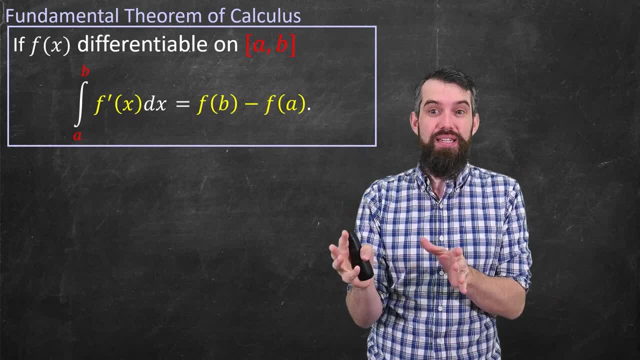 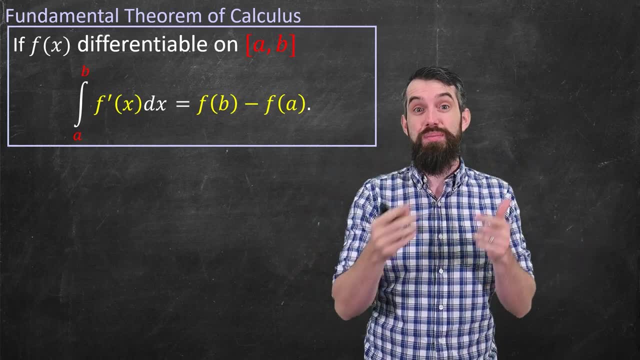 So really what we've seen is that that basic theme is consistent from the fundamental theorem of calculus back in single-variable calculus, up to the fundamental theorem of line integrals and then our big theorems of Green's Theorems, Part 1 and 2,. 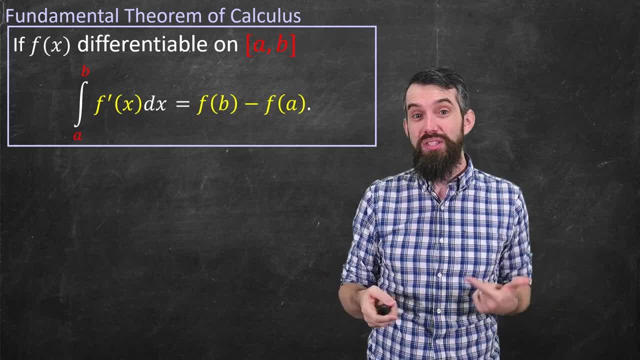 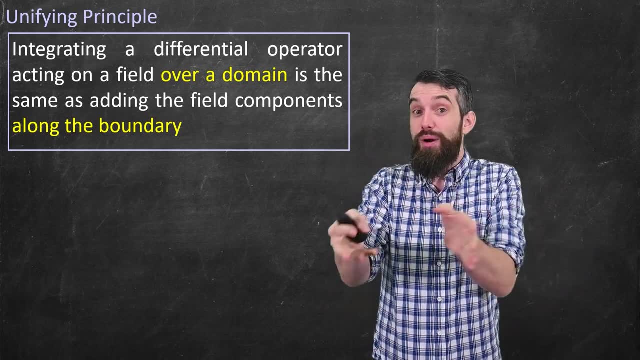 Stokes' Theorem and the Divergence Theorem. So, putting this all together, I'm going to write down a unifying principle which says: if I'm going to be integrating a differential operator over the entire domain, then this adds up to a measurement. 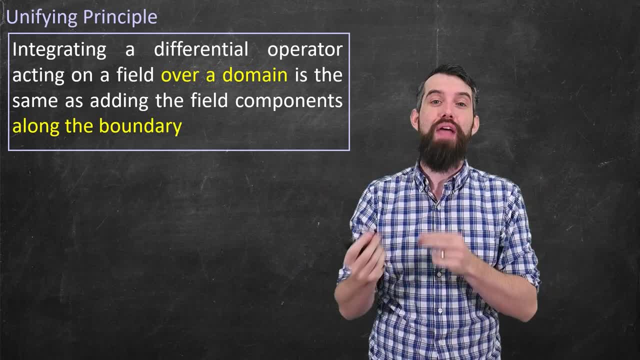 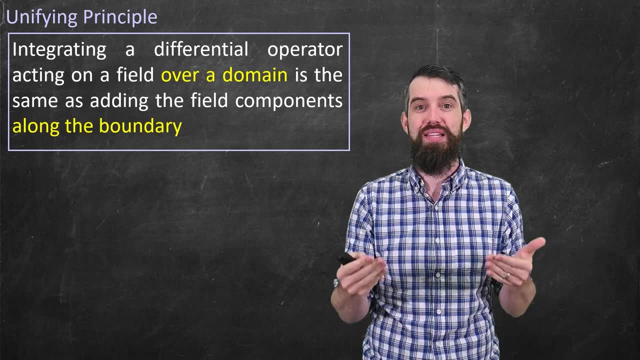 just to the dimension of f of b minus f of a, Just along the boundary of that domain. Exactly how you interpret this sentence depends on the context, As we've seen. we've seen a few different ways to interpret this, depending on what kind of object we're talking about. 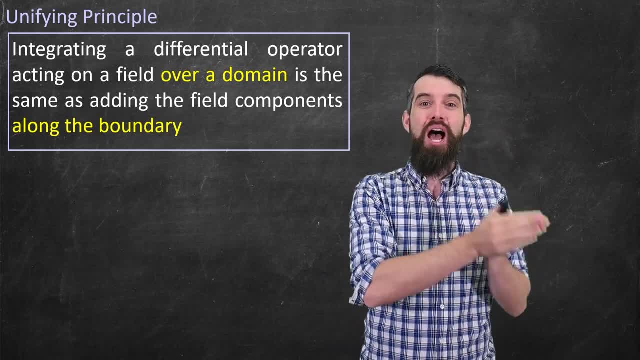 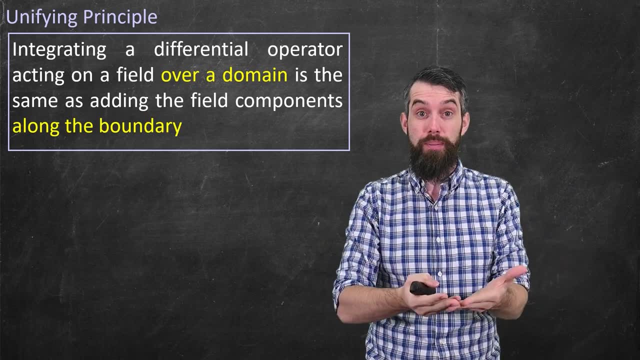 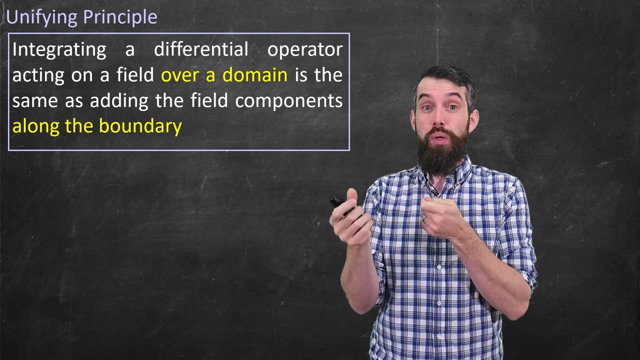 But the basic idea was always. this idea of adding up a differential operator over the entire domain gives us some information about just the boundary. And indeed, as sometimes we focus more or less on the proofs of these different statements, but all of them actually do rely on the fundamental theorem of calculus too. 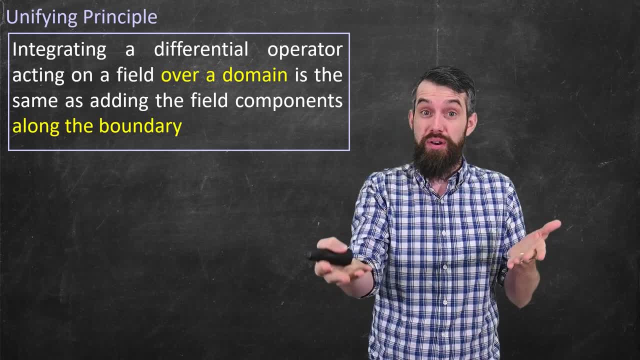 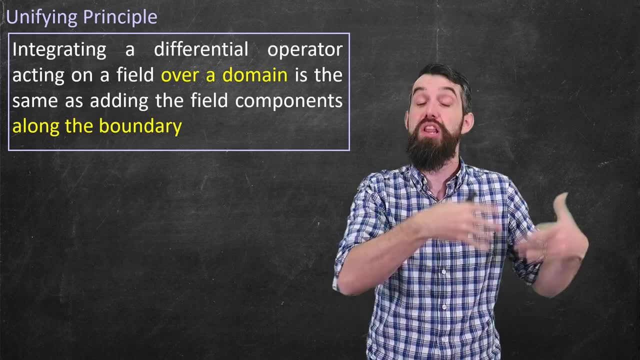 And one of the ways we can think about this is that all of these big, powerful theorems of vector calculus are different types of generalizations of the fundamental theorem of calculus, depending on what the context is. So you take the basic fundamental theorem of calculus too, and you generalize it to these different types of concepts.